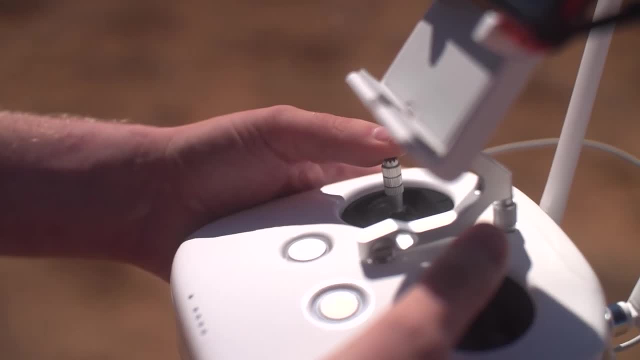 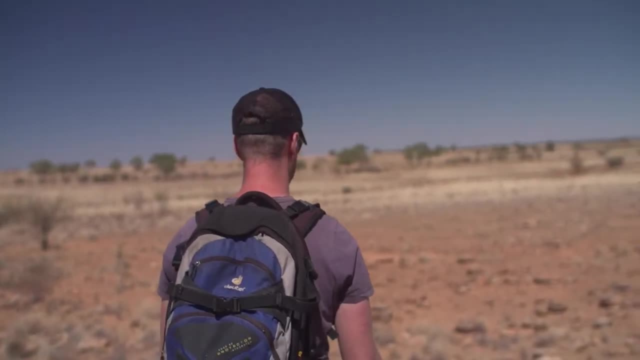 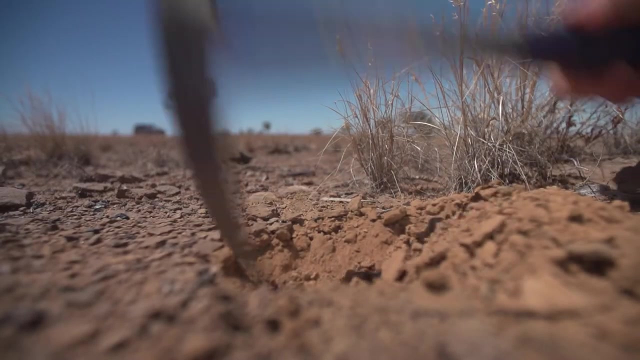 But it's still around 35 degrees and dusty and cold at night down to freezing temperatures. So sometimes when we find tiny little bone fragments, we follow them up the hill and we discover big things, like this big guy behind me here. So when we find the source of bones in the field, we start to dig a big hole. 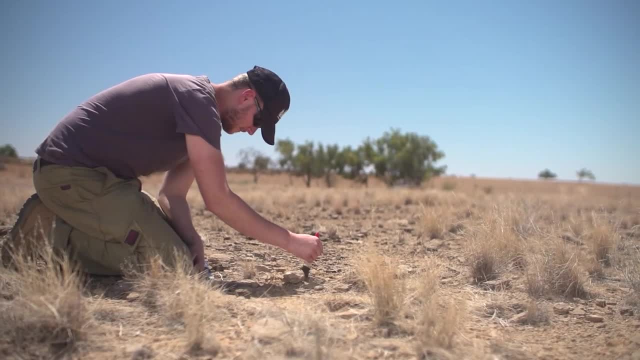 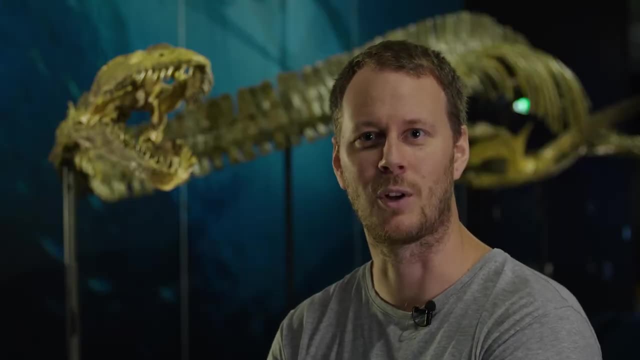 And if we're very lucky, we don't have to dig very deep and the bones are really shallow, so most of the time we'll only dig a hole that's about a metre deep. So part of being a paleontologist is to describe the fossils that we find. 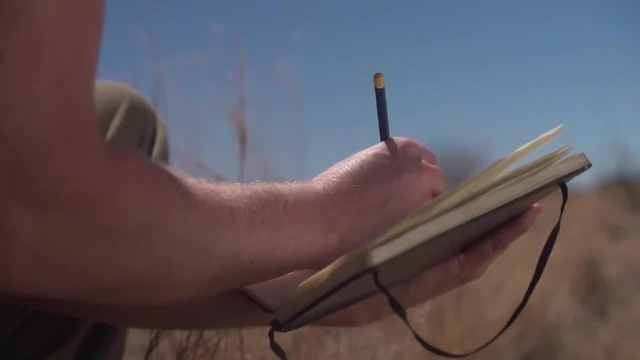 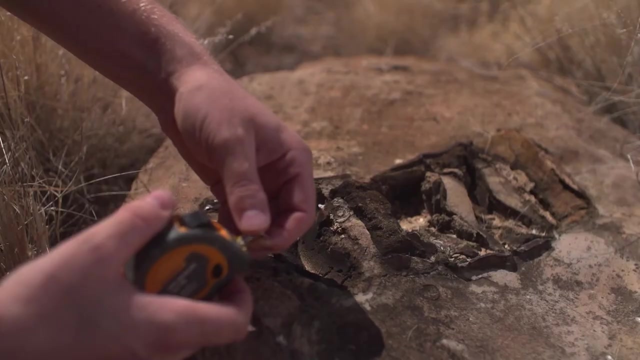 and by that I mean painting a picture for the reader of exactly what the anatomy of the animal looks like And describing the fossils are important because it allows us to compare them to other fossils across the world and find out what they mean to the evolution of life. 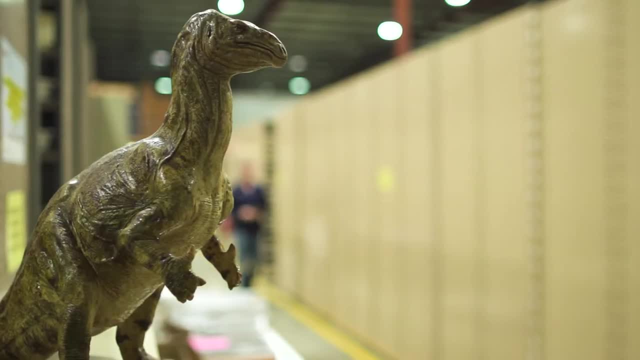 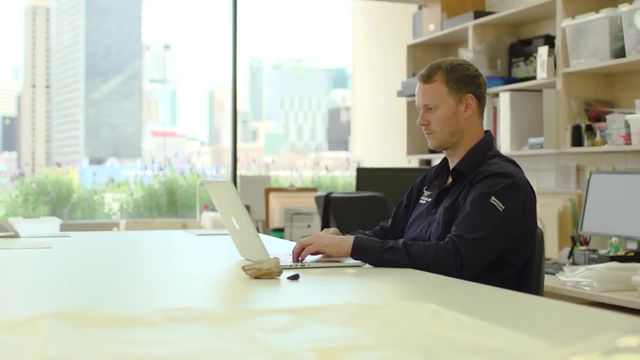 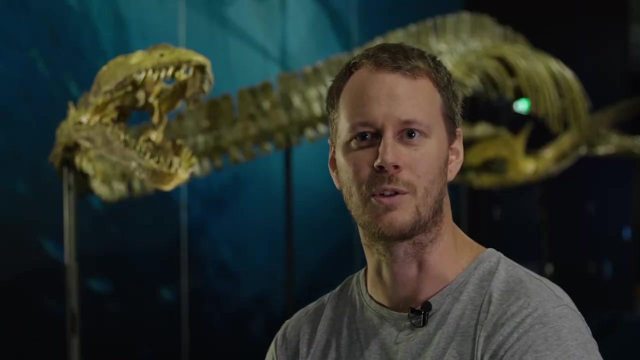 When we excavated the skeleton in the field and brought it back to the museum, we used a variety of technologies to study the animal. So we used 3D technologies that are some new innovative methodologies that have come in in the last few years. So using these 3D technologies, we're allowed to see inside the skeletons. 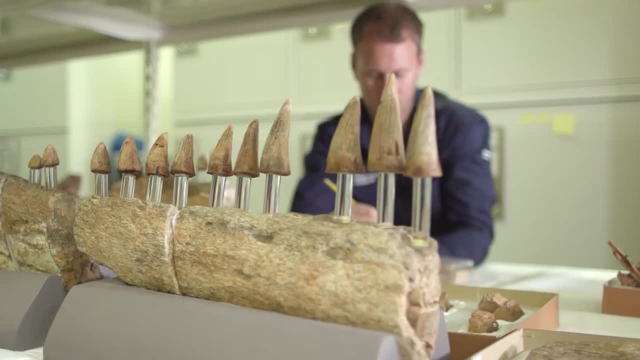 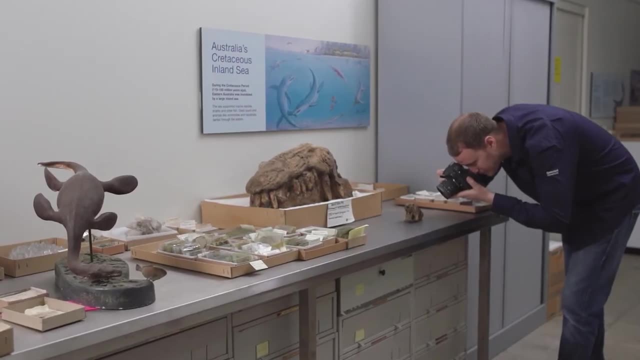 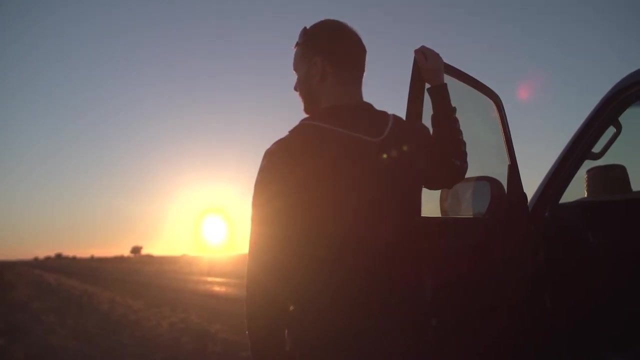 and also allowed to enlarge really tiny little bits of animals to better study them. Some of these 3D technologies include laser scanning and photogrammetry, and also micro CT scanning, which is X-ray of the fossils. As a kid, I remember always being interested in natural science. 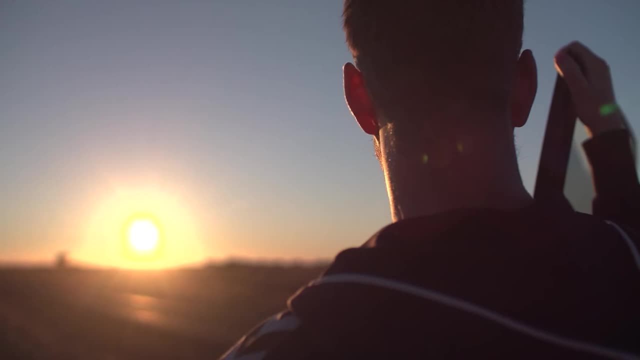 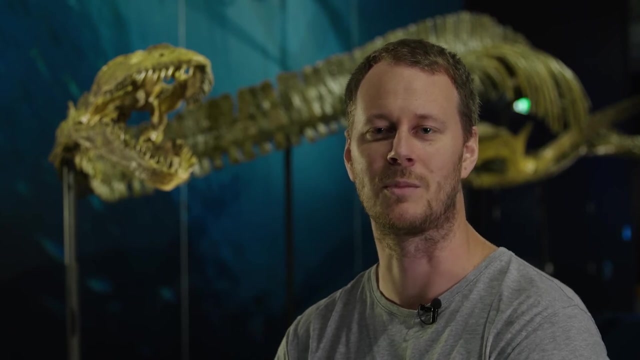 and I would go out and collect bugs in the forest and go to the local mines and collect rocks and minerals. I really fell in love with paleontology when I was up in the freezing arctic collecting ancient marine reptiles. We discovered over 30 skeletons of these ancient marine reptiles that were swimming around in this ocean 150 million years ago. 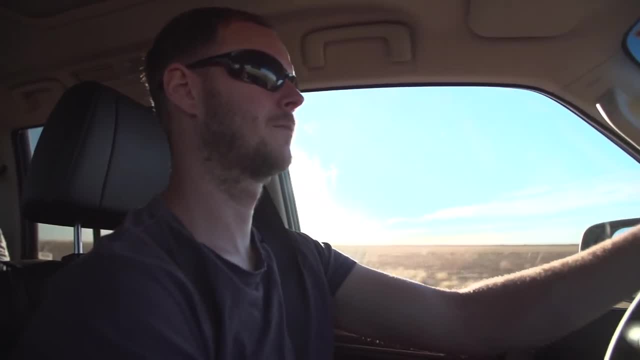 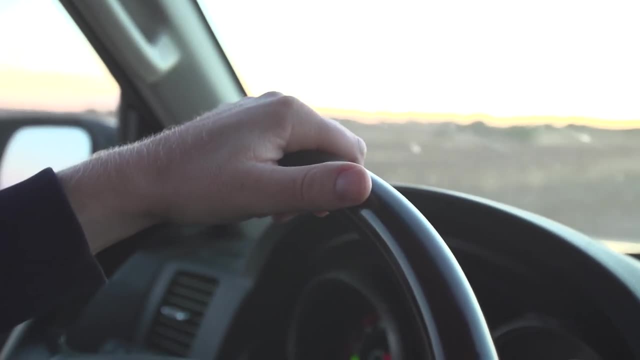 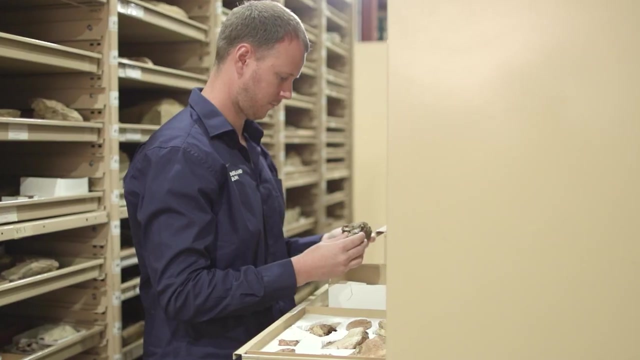 The discovery of all these ancient marine reptiles really made me think about our place in the world as humans and the ancient history of the earth. If you're interested in becoming a paleontologist, follow your dreams. go visit a museum, get in contact with universities and do all the science- subjects like biology and geology. 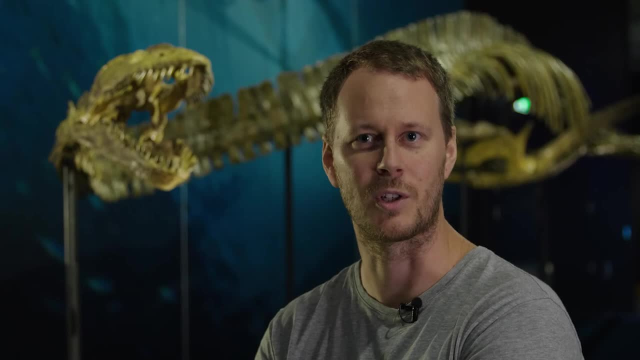 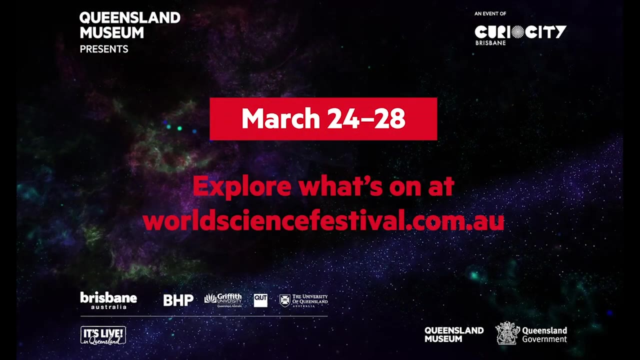 The ultimate question for me and for my work is: what is the origin of life? How did it evolve and how did it end up where we are now? Find out more at wwwpaleontologycom.